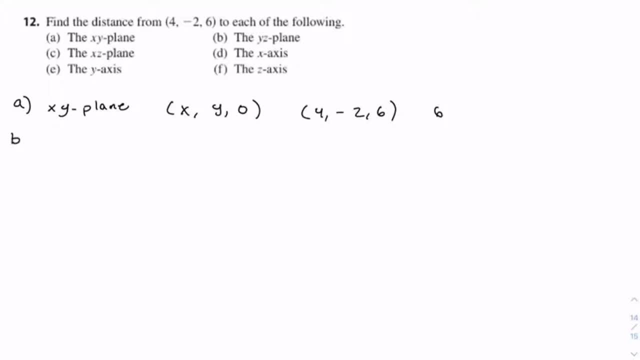 That's the distance. So we just want to look at the x component, which is 4.. And 4 is 4 units away from 0. So that's the distance for, say, 4 units, Because it doesn't specify anything else. See, We have the xz plane And that happens when y is 0. And x and z can equal anything. So if we compare to our original point, just like before, the x and z can equal anything. 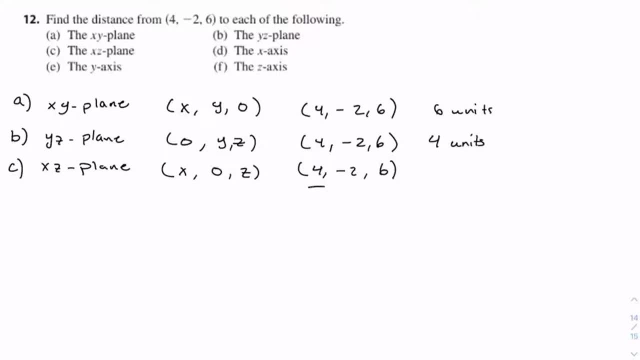 The x and z component do not matter, So we can just compare to the y And since negative 2 is 2 away from 0, when I say 2 away, I'm referring to the absolute value of magnitude, Because distance can't be negative. So we have 2 units. 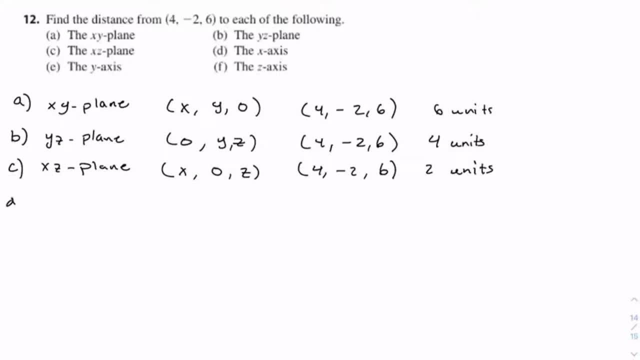 So now try to think of how could you represent the x-axis for part d in points that are bounded and not bounded. So if you got that x was bounded, not bounded, and the y and z components had equal 0,, you got it right. So x can equal anything, but as long as the y and z equal 0. So instead of having 1 value that we need to compare to find the distance, we have 2.. 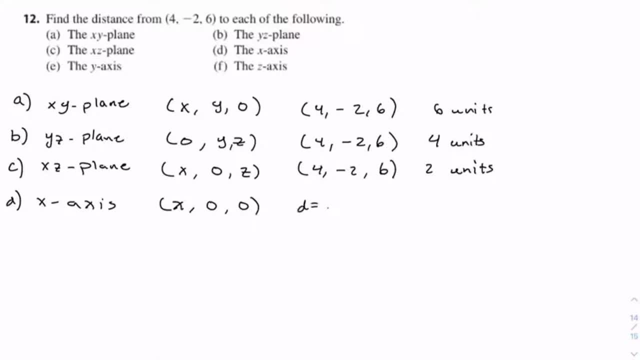 So this requires the 4 units. This is the distance formula for 2 components: x minus x1 squared plus y minus y1 squared. And these x's and y's don't correspond to these. Well, here I can make them correspond. 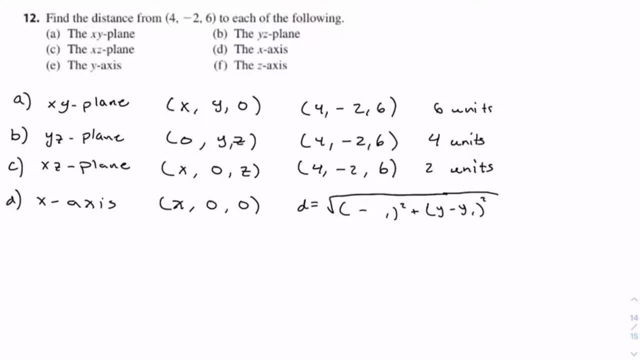 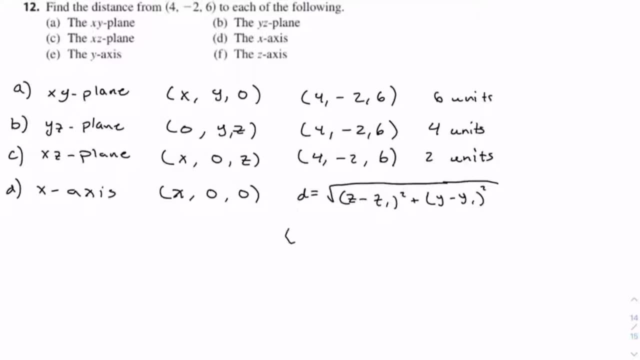 Instead of being x, we can just make this z, But these just represent 2 points that are away. So we have the 4, negative 2.. Let me do this in a different color. Let's do this entire problem in a different color. 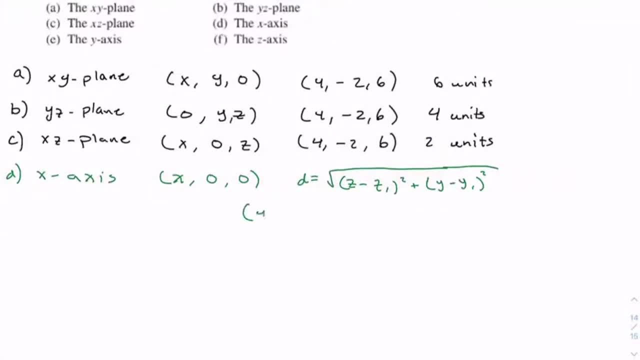 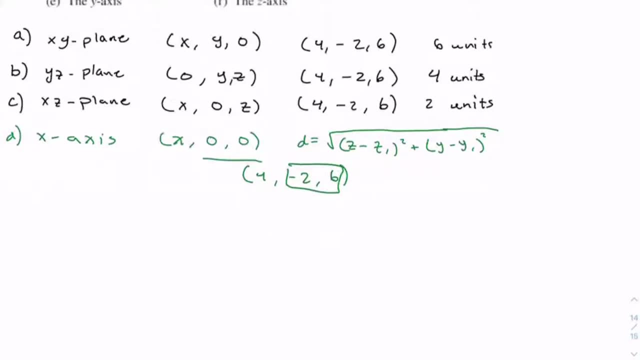 Because x can be anything. We're just looking at the 2, negative 2 and 6 at this point. So we're just looking at these 2. And we're comparing it to 0, 0.. So we have the d equals 6 minus 0 squared plus. 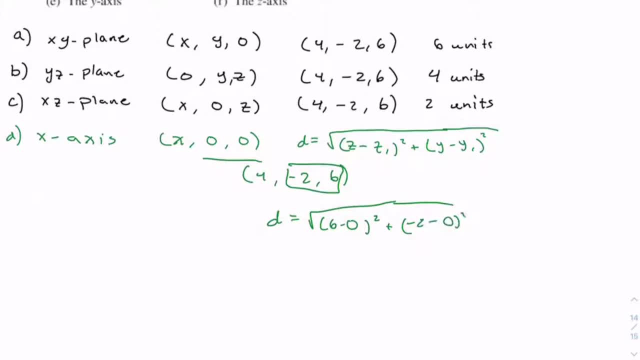 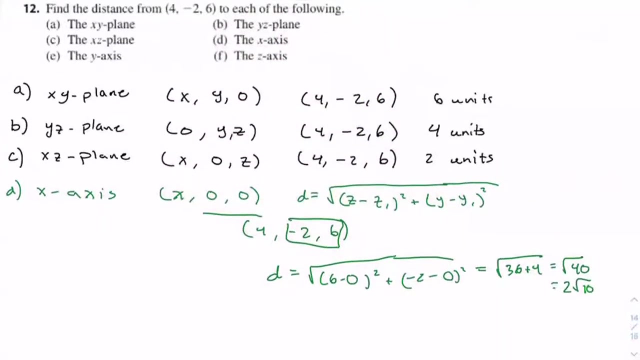 Negative, 2 minus 0 squared, Which equals square root of 36 plus 4 square root of 40. That equals 2 root 10.. So now let's go on to part e, which is the y-axis, And the y-axis can be bounded by 0, y. 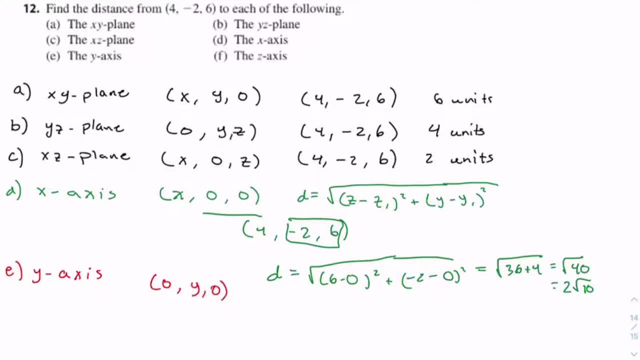 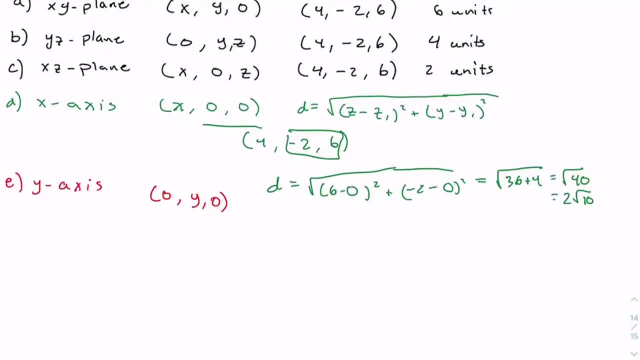 0, y being any point, And this creates the Y-axis. So, just like earlier, we use the distance formula for x and z. So, rather than this being z and this being y, We're going to just use x and z. 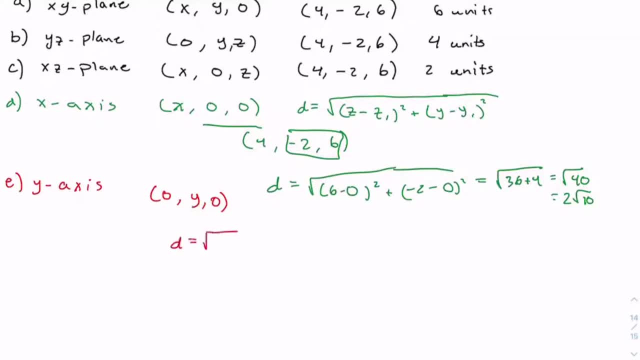 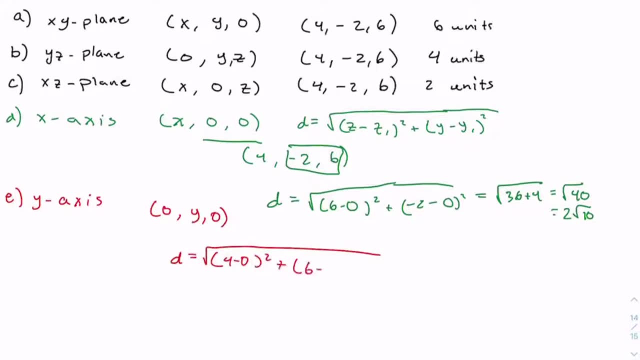 So we have: the distance equals 4 minus 0 squared Plus 6 minus 0 squared. This equals square root of 16.. Plus 36. Which equals square root of 52. See if you can simplify this at all. 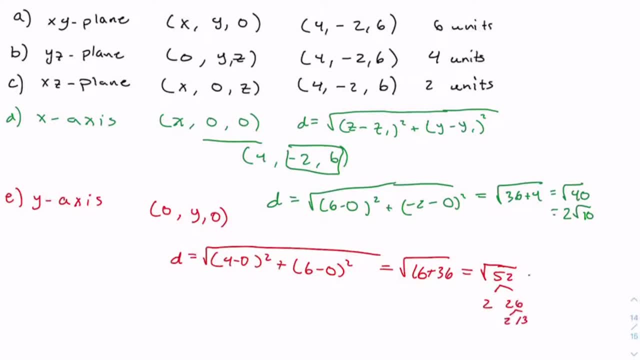 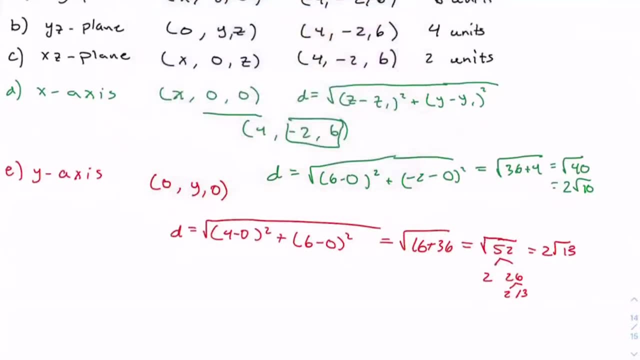 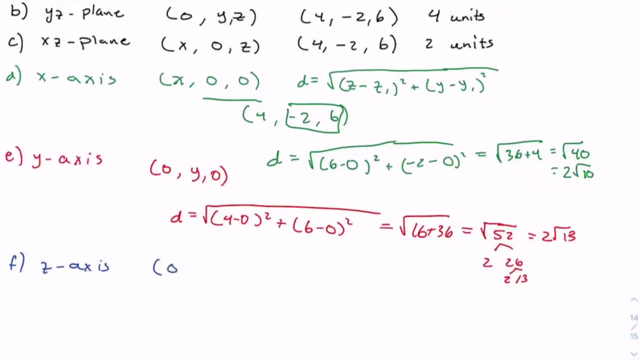 2, 26.. 2 and 13.. Equals: 2 root 13.. Then, for the final part, F, We have the z-axis. This can be represented by 0, 0, z, Z being any number. 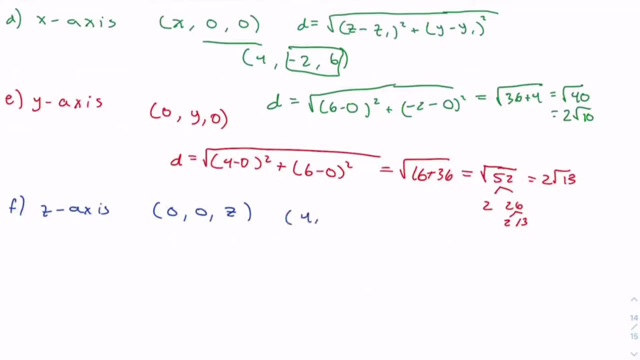 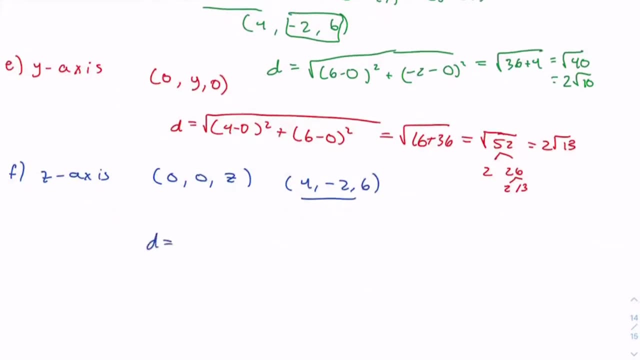 And just to write it down again, Our point is 4, negative 2, 6.. And we're just going to keep comparing the x and y component So we can say the distance Square root of 4 minus 0 squared. 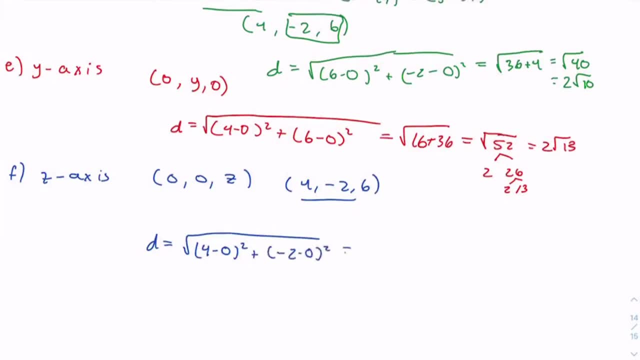 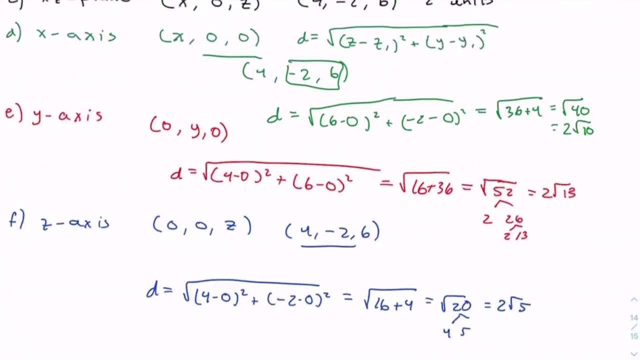 Plus negative 2 minus 0 squared, Which equals 4 squared 16. Negative 2 squared, which is 4. Square root of 20. We get 4 and 5 equals 2 root 5.. So these are the three distances.